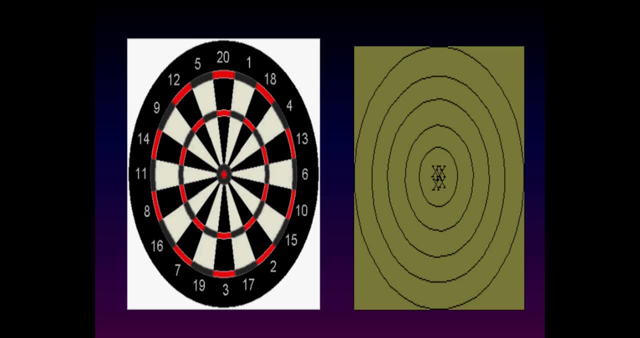 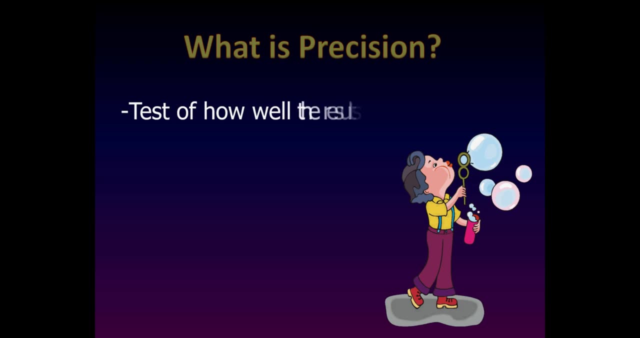 put that into a real-life situation, for example, this dartboard: our target is the bull's eye. So if all the dart pins will hit the bull's eye, definitely we are accurate. What is precision? Precision is number one test of how well the results agree with one another. 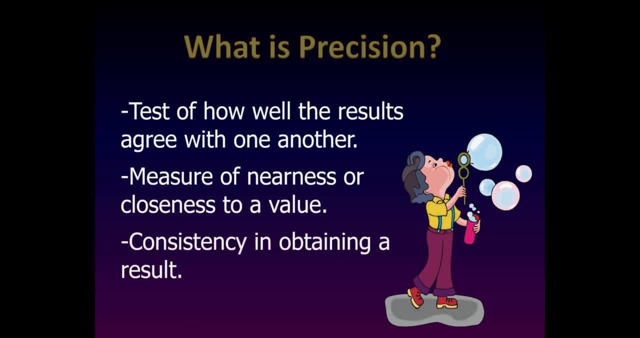 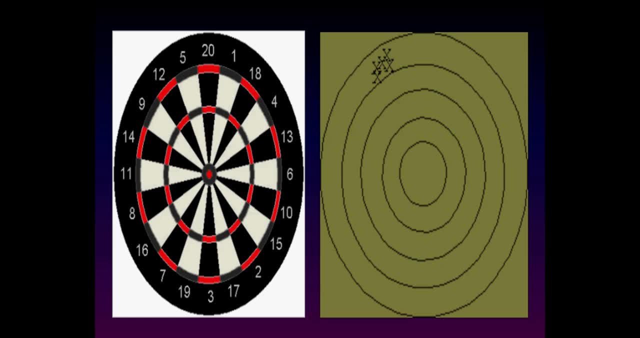 Next, measure of nearness and closeness to the value And lastly, consistency in the obtaining of the data. Let's put those definitions in this sample diagram. So if you will notice if this is the dartboard and all the dart pins was placed or was targeted on this certain point. 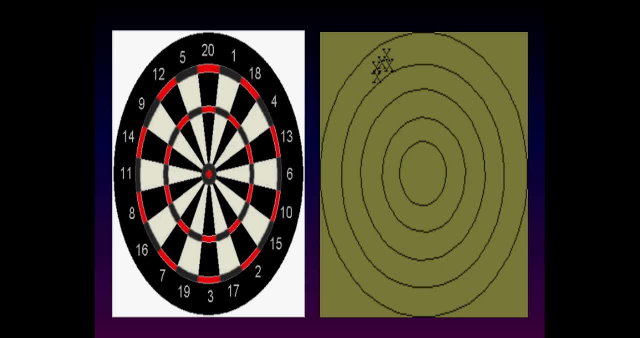 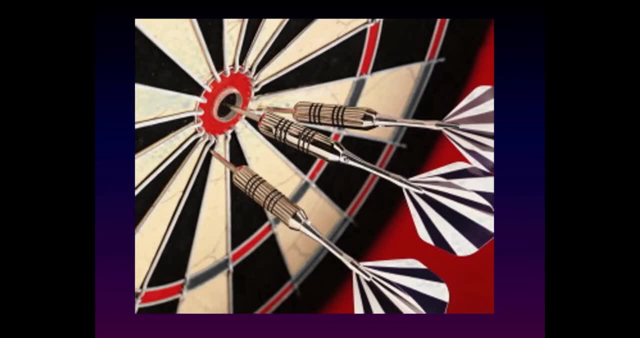 definitely you are not accurate, but you can say that you are precise because all of the dart pins are very near from each other And let's have this one. So if you will notice, in this dartboard, one of the dart pins are hit. 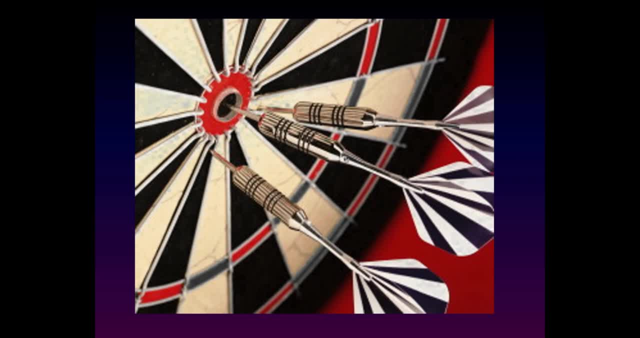 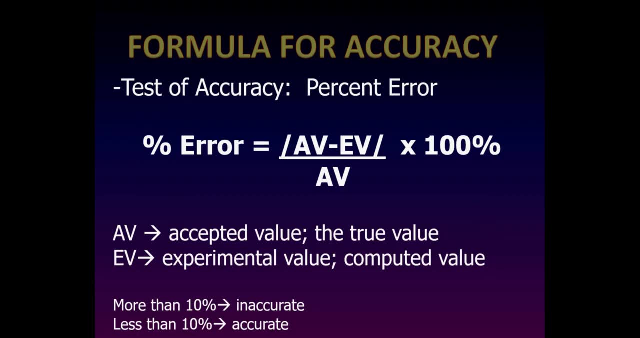 hit at the target, while the other two did not. So therefore, we can say that we are accurate but not precise In the build up science where, in you are going to test the values that you obtained, you can use the test of accuracy or the percent error. 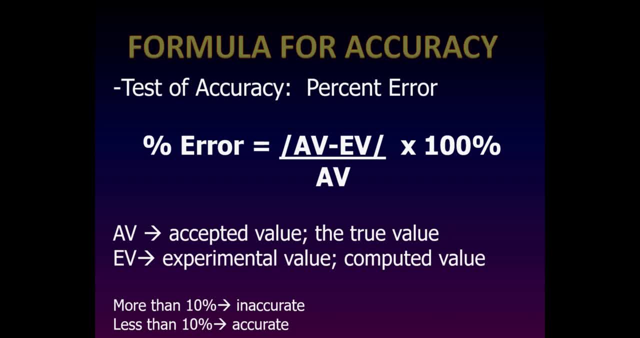 This is the formula for the percent error. Percent error is equal to the actual value minus the experimental value, which is the absolute value of it over the actual value times 100%. If your value is more than 10%, We can say that you are inaccurate. 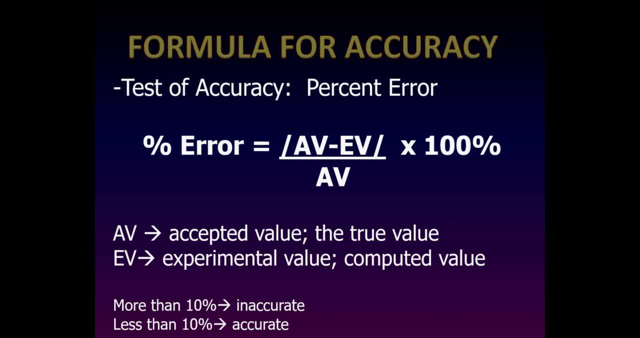 But if that is less than 10% you can say it is accurate. But this is only just applicable for us in our school, But in some universities sooner, or even in your field, if you're going to choose Med-Tech or even other courses in college. 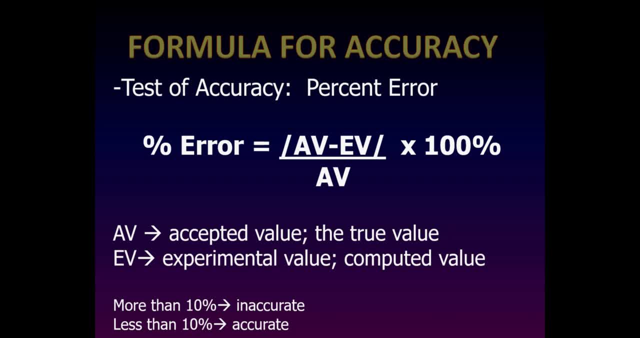 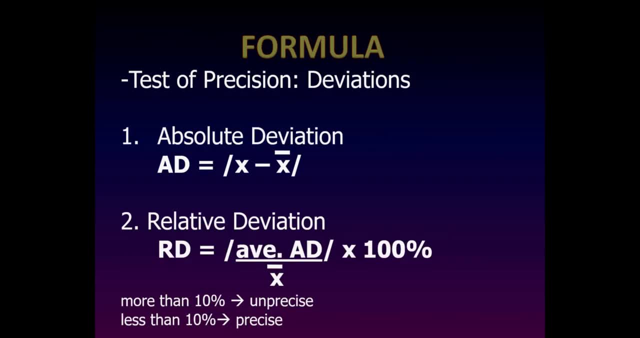 you might encounter this and they might have different set of agreement for the accuracy- accuracy of the value. the test of precision is known to be the deviations. so when we are talking about deviation, this actually the absolute deviation, wherein it is equal to the x minus the x bar. 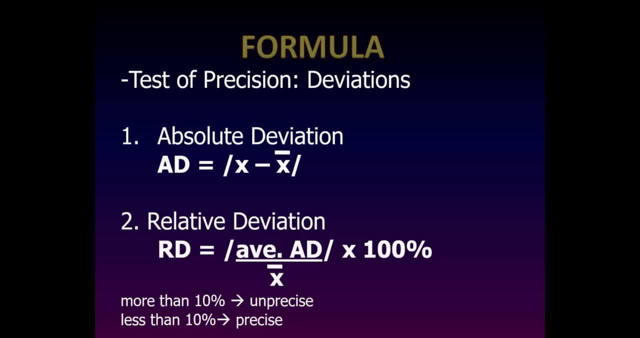 and the relative deviation, which is actually your average absolute deviation over the mean value that you obtained, times 100. if your value is more than 10 percent, you're unprecise, but if that is 10 percent or less, that will be precise for us. again, it is only applicable in our 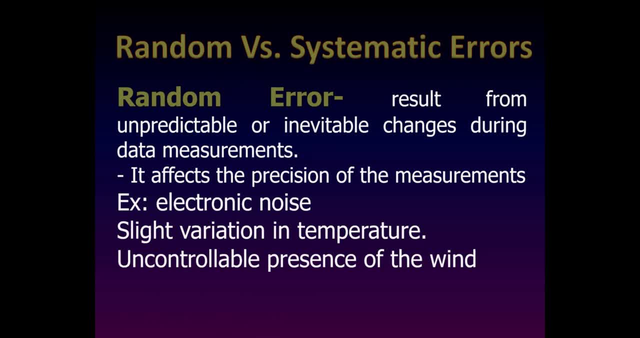 school. as i said to you a while ago, in our objectives we are going to differentiate random to a systematic errors. so in the field of science there is no perfect result, but there are a reason. why do you obtain, or you have obtained, those kind of errors in your result? so when we are talking about random error, this is the 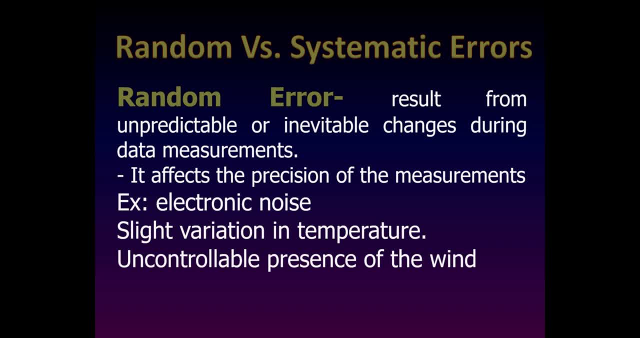 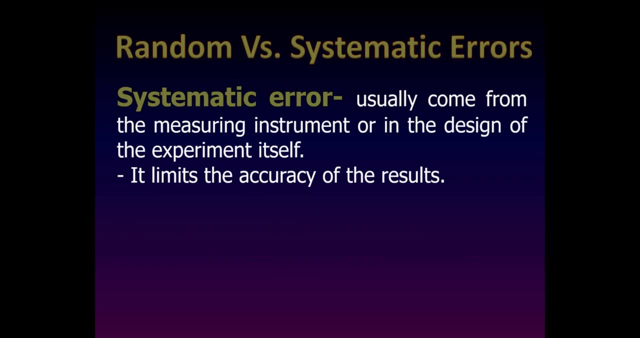 result unpredictable or an evitable change during the data measurements. it affects the precision of the measurement. example is the electronic noise, slight variation in temperature and uncontrollable presence of the wind. another type of error is the systematic error. usually come from the measuring instrument or in the design of the 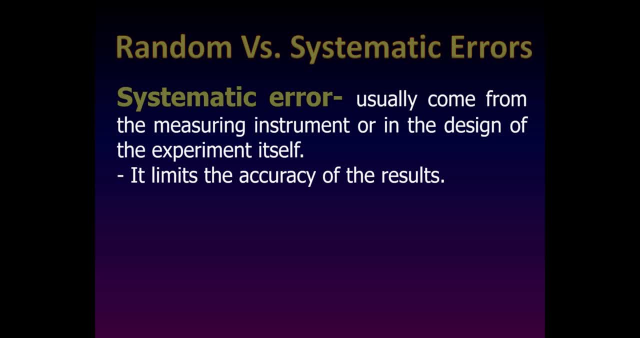 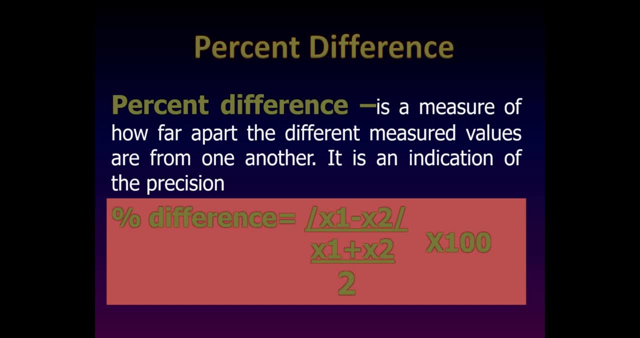 experiment itself. here, it limits the accuracy of the result. aside from that, we can use the percent difference when we are talking about percent difference. this is the measure: how far apart different measurement values are from one another. it is an indication of the precision, so for you to solve for it. this is the 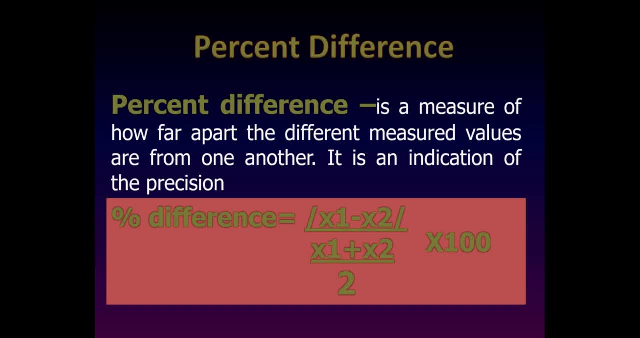 formula for the percent difference. percent difference is equal to the measurement 1 minus measurement 2 divided by the measurement 1 plus measurement 2 over 2 times 100. this is used for you to determine whether the values that you obtained, the two values that you 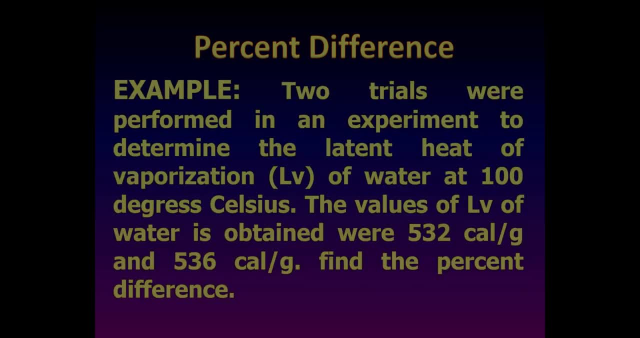 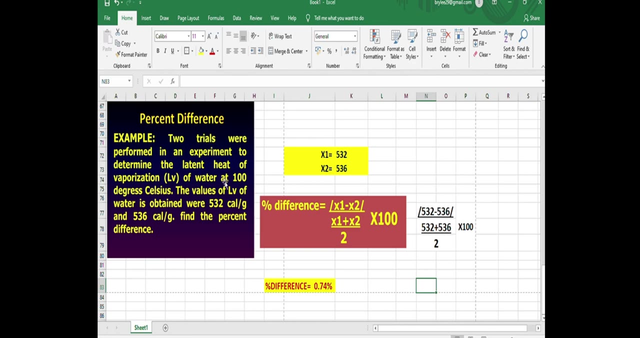 obtained is precise for this example problem for percent difference. you will see the complete solution of the answer on the next slide. for some let's try to solve the percent difference sample problem, but before that let's read. so two trials were performed in an experiment to determine the latent heat. 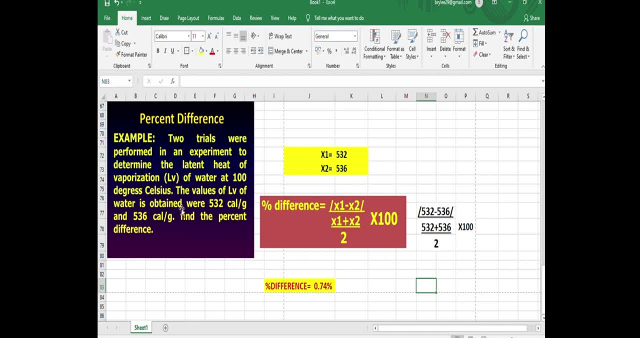 of vaporization of water at 100 degrees celsius and the temperature at 100 degrees celsius, the values of lb of water is obtained were 532 calories per gram and 536 calories per gram. find the percent difference of the value. so x1 is 532. 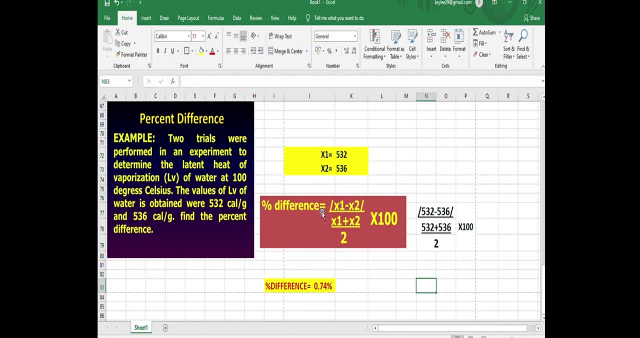 and our x2 is 536. using the formula for percent difference, which is x1 minus x2, the absolute value divided by x1 plus x2 divided by 2 times 100, so the result is 532 minus 536. we will get negative value here, which is: 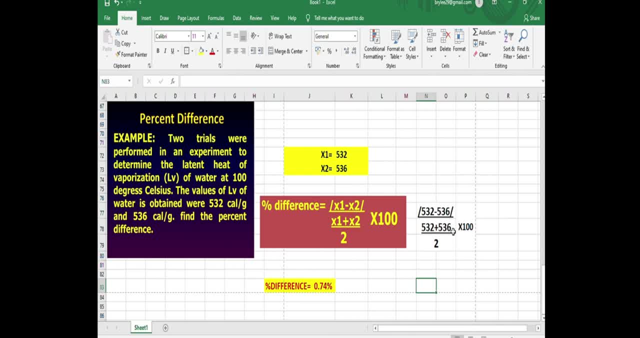 negative. 4 divided by 532, plus 536 divided by 2, then multiply it by 100, we will get 0.74 percent. so therefore there is a 0.74 percent of percent difference between the two values obtained in the experiment. let's try to solve the percent difference. sample problem. 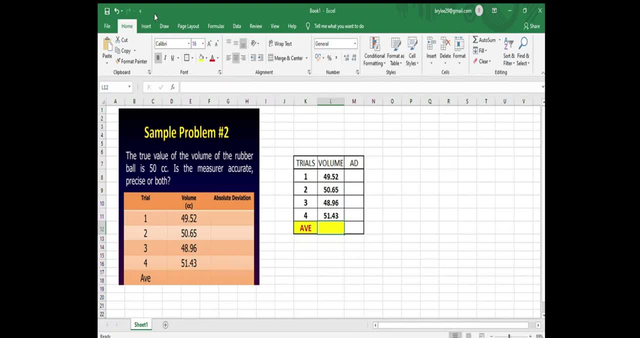 but before that let's read: let's solve sample number two using microsoft excel. so, for example number two, let's read first the problem. the true value for the volume of the rubber ball is 50 cc. is the measure accurate, precise or both? so here i will be showing you how to. 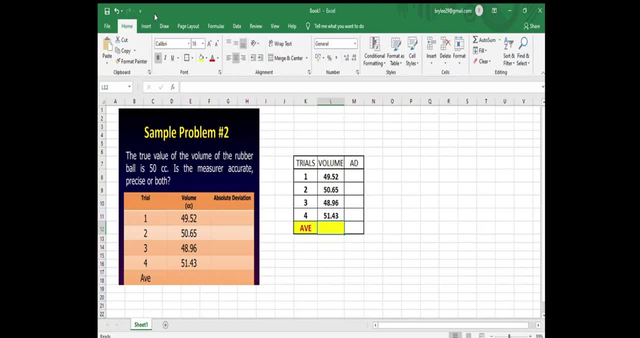 solve for the average and the absolute deviation. so i have written here the trials that we have: one, two, three, four. so we have four trials and the value of the volume per each trial. so we need to solve for the average volume. so how do we do that? so right here. 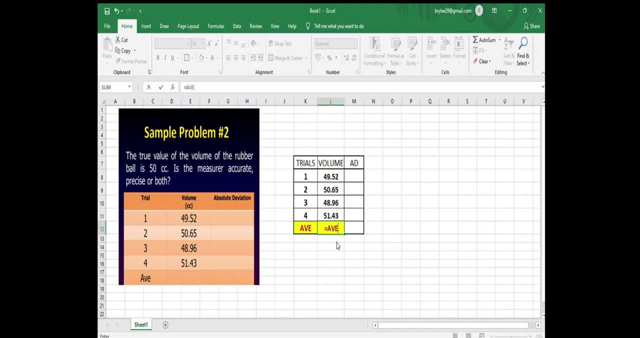 equals, then average the word average open, close parenthesis. then drag the value that you have here, then close parenthesis, then press enter. so there you have it, so 50.14. now how do we solve for the absolute deviation? so, for the absolute deviation, as we all know, this is the difference between the 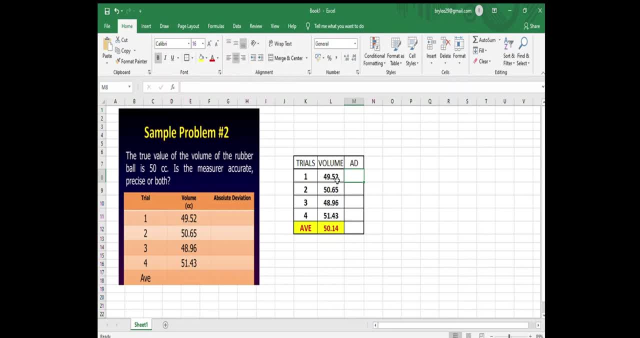 average volume minus the value obtained for each trial. so you just write equals, then 50.14 minus l8, then press equals, so we have 0.62 for the first trial. then then let's drag it here to the fourth trial. then you have the value for the absolute deviation. 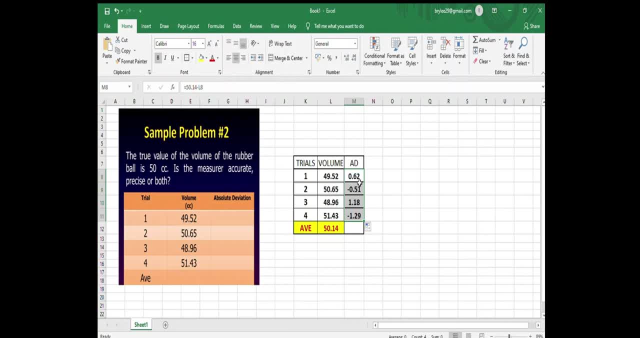 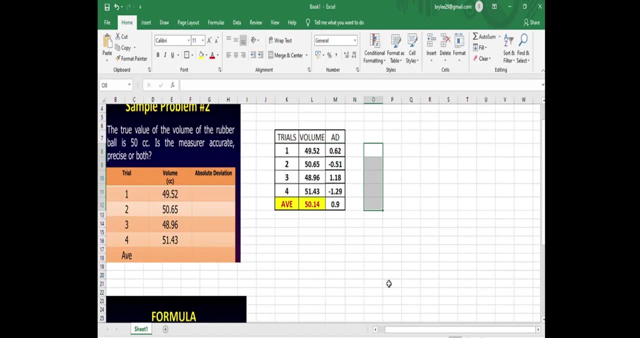 but since it's absolute deviation, we are going to disregard the negative sign in getting the average absolute deviation, since we're done already solving for the absolute deviation value. and, as we all know, for getting the average absolute deviation, what are we going to do is to copy the values that we have here for trials one. 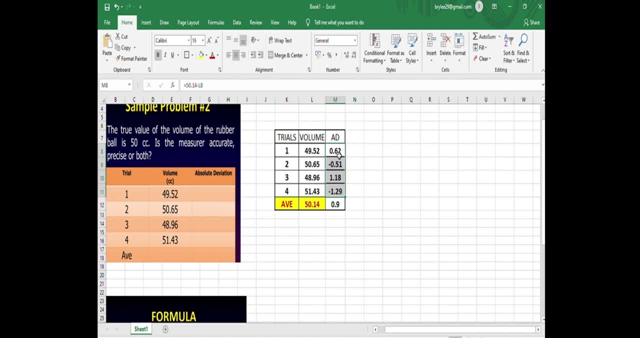 to four for the absolute deviation. so let's copy the value. so right click, then copy, paste it on the other side, then paste values. so with that, as you all, as you can see, we're just going to remove the negative sign for trial 2 and trial 4.. so that we can solve for the absolute. 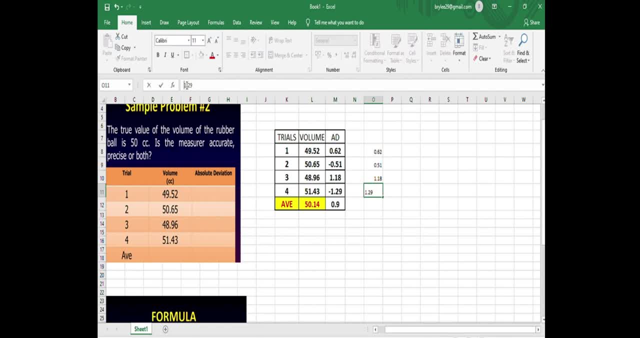 absolute deviation. so with that then let's remove, then below let's try to solve for the average absolute deviation. so if you have Equals, then type the word AVERAGE, then open, close parenthesis, then drag from this 08 up to 011, then close parenthesis, then press ENTER. 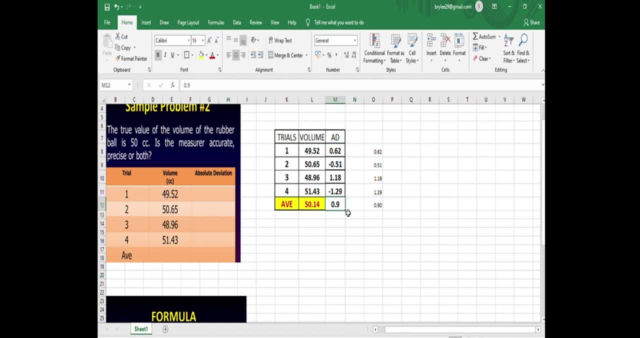 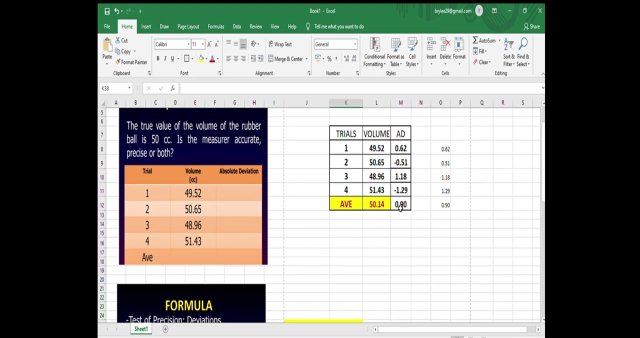 Then you will see the answer will be 0.90, which I place it here on this part, so 0.90.. So let's just increase the decimal places. Since we computed already for the average volume together with the average absolute deviation, we can now solve for the precision of the values that we have. 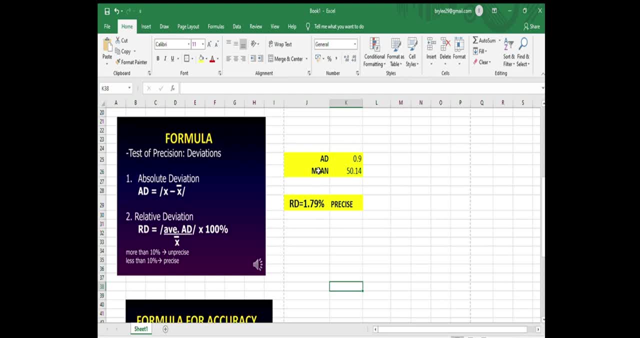 So, for the precision, we're going to use the absolute average deviation together with the mean value. So using the relative deviation formula, which is average absolute deviation divided by the mean value times 100.. So using the value, so 0.90 divided by 50.14 times 100, you will get 1.79%, which is precise. 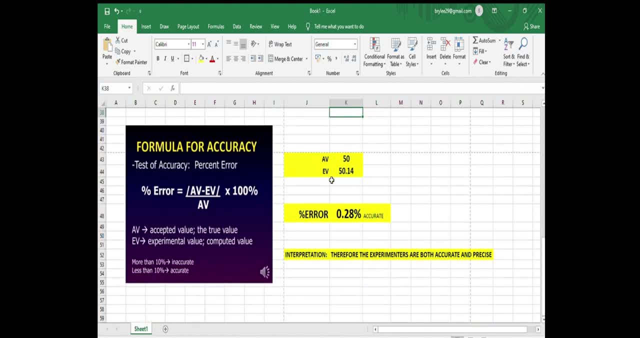 Next, for the percent error, you're going to use the actual value for the volume, which is 50, and the experimental value, which is 50.14.. So, using the formula AV minus EV divided by AV times 100..